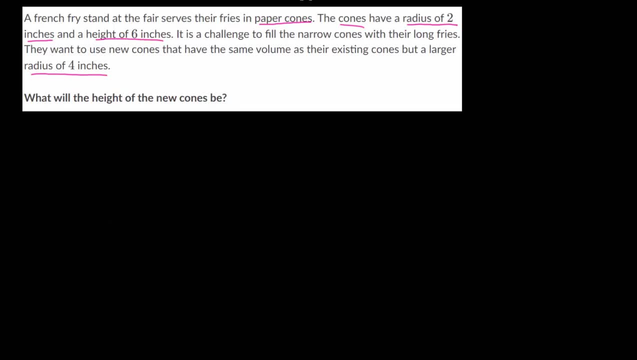 And before we try to answer this, let's just draw a picture of the shape that we're dealing with, Since we know we have a cone and remember that cones have circular bases and they're not circular. So let's draw a picture of the shape that we're dealing with. 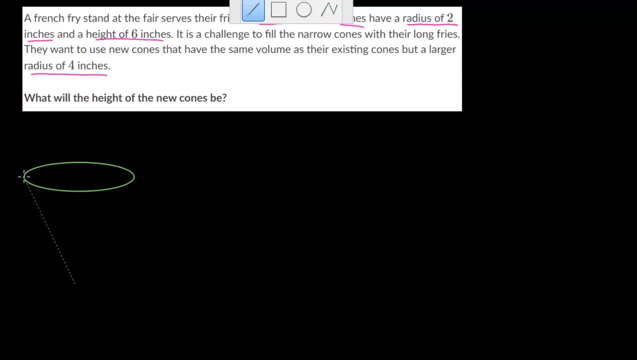 And before we try to answer this, let's just draw a picture of the shape that we're dealing with, And every point on the edge of the cone will meet at a point either above or below the circular base. And again, we can draw these lines from any point on the edge. So maybe, 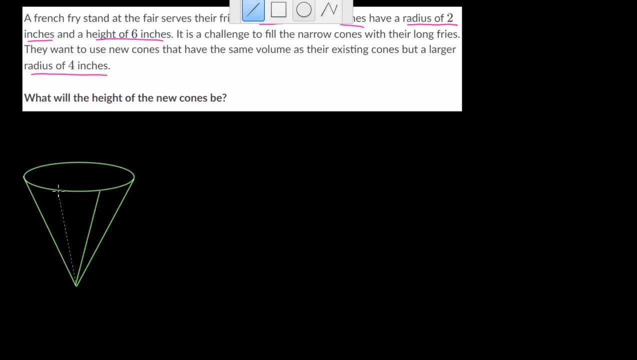 from here or from here, it doesn't matter. They will all meet at this bottom point And what we're told is that we're going to use a larger cone than the one they originally used, And the original one had a radius of two inches and this one will have a radius of four inches. 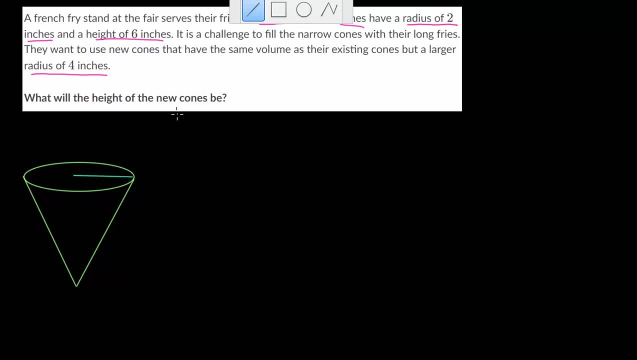 So the radius that they're referring to, that is the radius of the base. And again, the radius is just the distance from the center of the base to the edge of this circle, And it's four inches. Now we need to find the height of this new cone And what we're 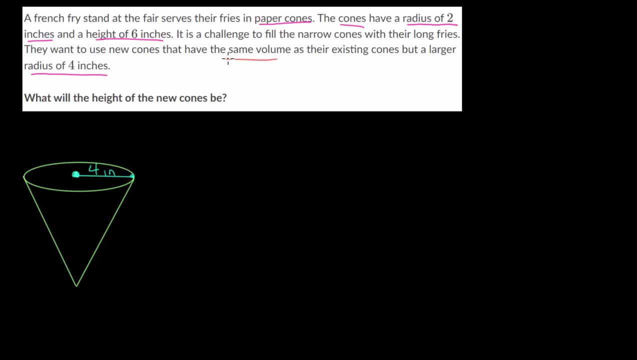 told is that the new cone has the same volume as the existing cones. So let's draw another picture of the initial cone that they were using, And we know that cone will have the same volume but a narrower radius or a smaller base. So this cone will likely be: 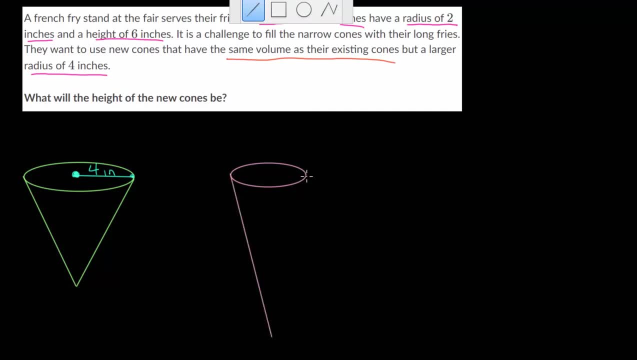 much taller so that they can have the same volume. They take up the same amount of space. And this isn't going to be drawn exactly right, but we can at least get a rough idea. And we know the radius of this cone. This is two inches. 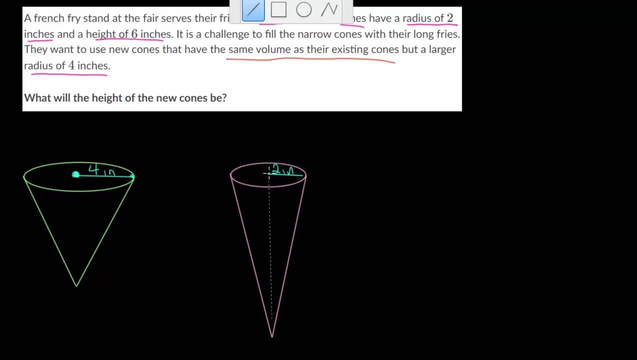 And we're told what the height is. The height of this original cone is six inches, So we can mark that in And remember the height. we can call that H is perpendicular to the base and runs all the way to the bottom. 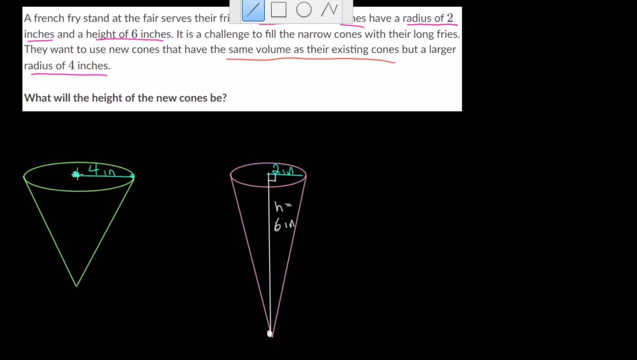 bottom point here, So we can also draw the height in for this cone, and that's what we're trying to find. So let's call this height h1 and we can call this height h2, and for our radii, we can call this r1 and this one r2.. Now to figure this out, we need to figure out the volume of this original cone. 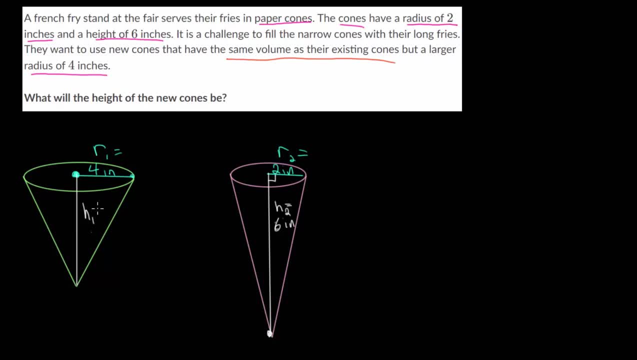 and use that volume to figure out the height in our new cone. But remember the formula for the volume of a cone: that it's equal to the area of the base of the cone multiplied by the height and then divided by three, Or it's one-third of the area of the base which, since it's a circle, 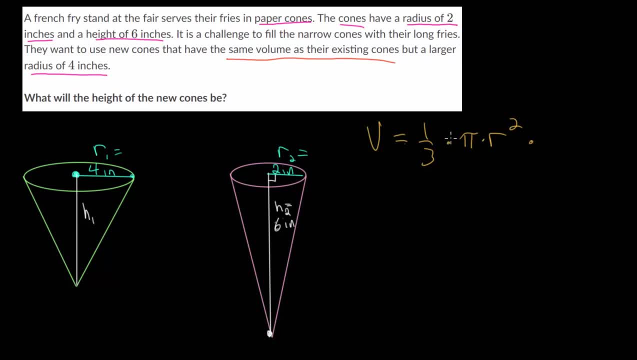 it will be pi multiplied by the radius squared and then multiplied by the height. So let's figure out the volume of the cone. So let's figure out the volume of the cone. So let's figure out the volume of this original cone and we'll use that to figure out the height of our new cone. So let's. 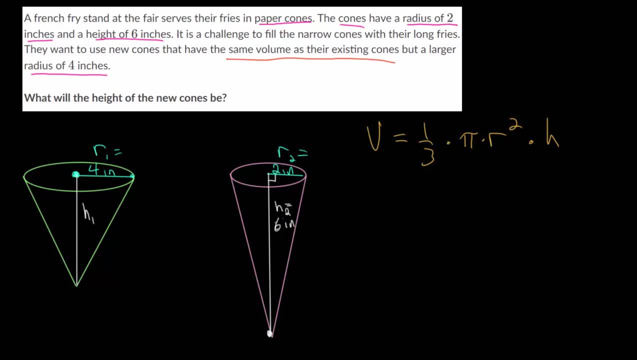 just start plugging in our numbers. We have that for this volume, which we can call v2, since we're using the subscript of two for this cone. This is one-third multiplied by pi, multiplied by the radius squared. So that's two inches squared multiplied by the height, which is one-third. 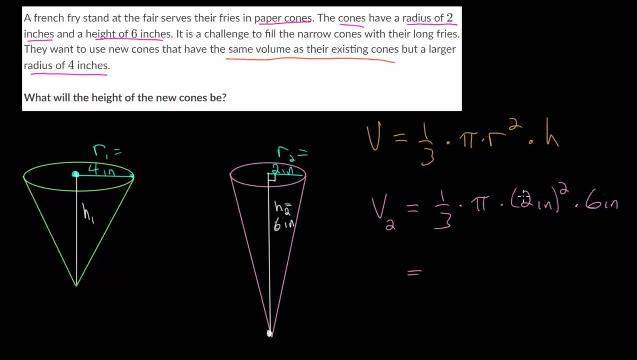 which is six inches, And if we simplify everything, this is four square inches times six, So that would be 24.. And we have square inches times inches, which will be cubic inches. We'll divide that by three and multiply by pi, And 24 divided by three is just eight, So we have eight pi And again we're. 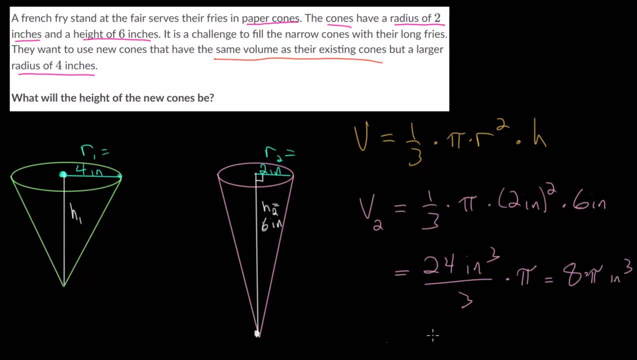 dealing with cubic inches here. So that's the volume of the original cone and it's the volume of our new cone. So let's use this information to figure out what the height will be in this new cone And we can say the volume of this cone. eight pi cubic inches is equal to one-third.